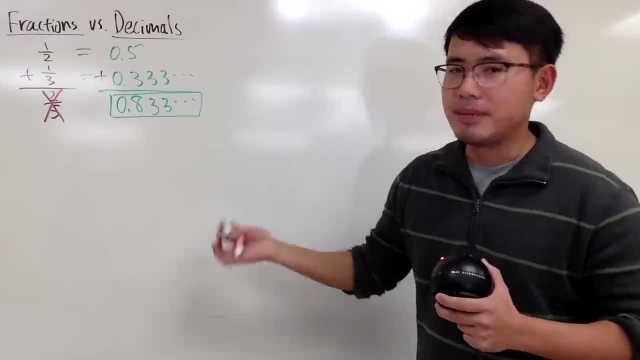 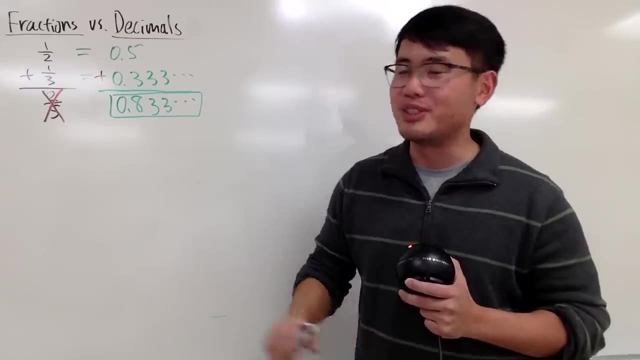 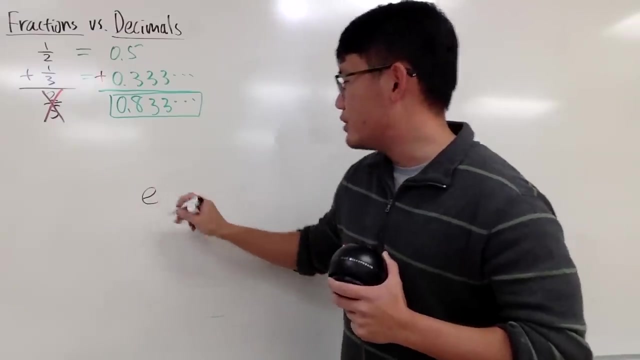 So decimals are much better. And why am I telling you guys this? Well, as I said, decimals are much better, but it's not easy to get the decimal expansions of some bad numbers or complicated numbers. Why not Imagine if you have to do e plus square root of 2.. 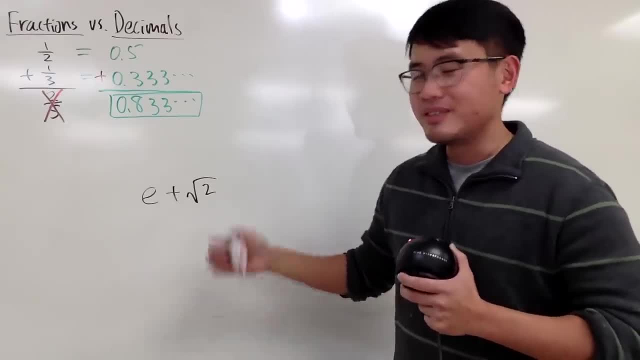 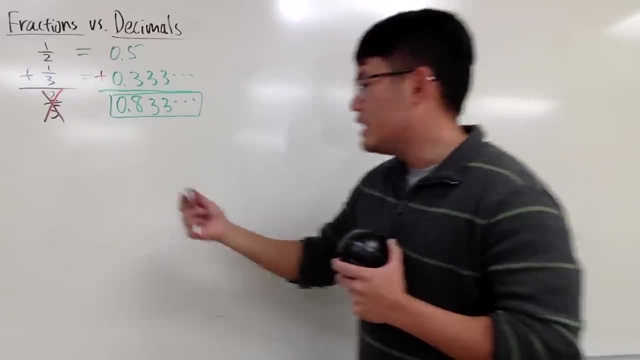 You have to figure what e is and you have to figure what square root of 2 is for decimal. It's not so easy, But I do have some videos on these numbers already so you guys can check. Anyway, this is still a calculus video. 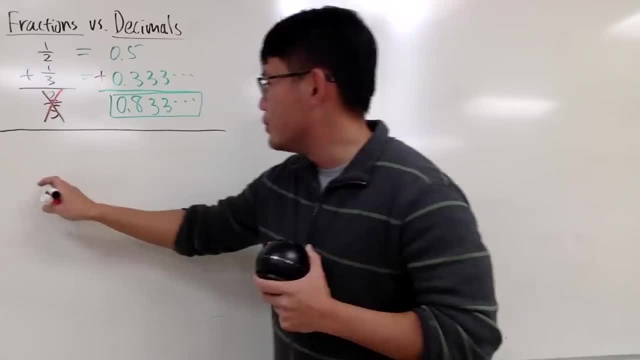 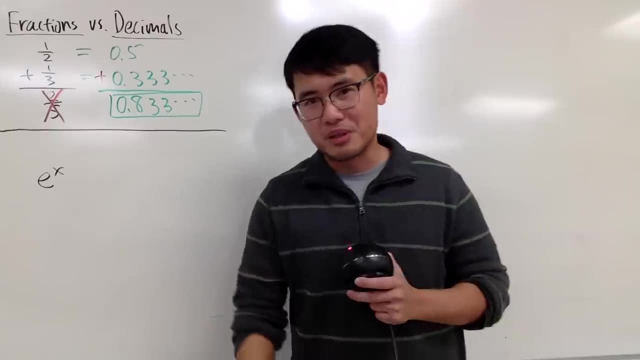 The idea is the following: What if, today, I want you guys to add two functions, Maybe e to the x? This is a common function that we have to talk about in calculus, of course. And then let's add another one: 1 over 1 minus x. 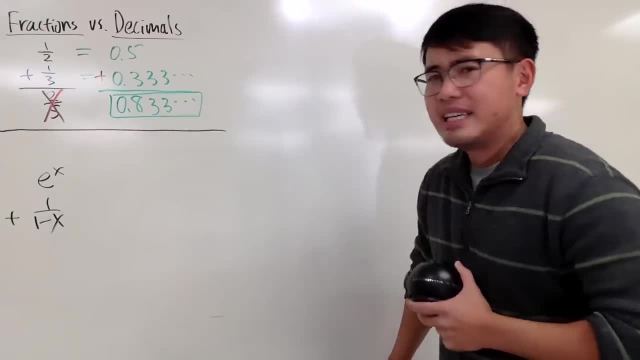 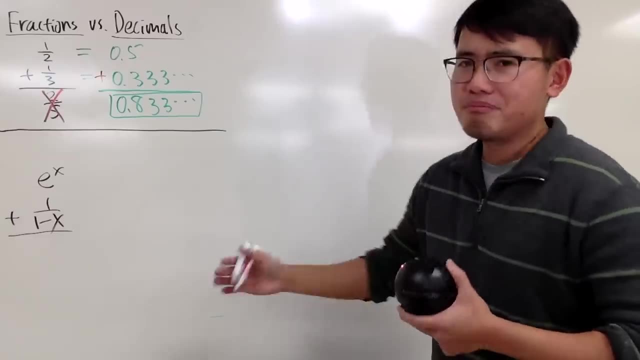 Okay, e to the x plus 1 over 1 minus x. I cannot do anything. Maybe get a common denominator. I can do all that, but yeah, that's about all. Or maybe e to the x plus sine of x. 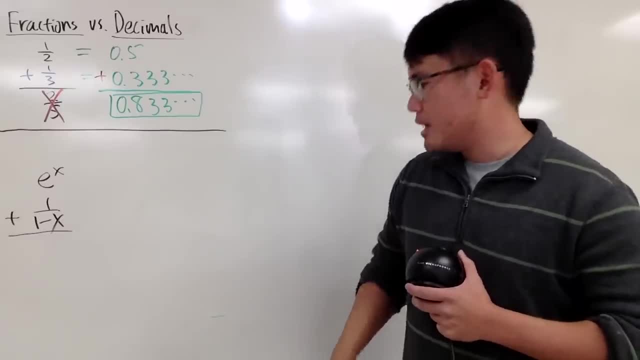 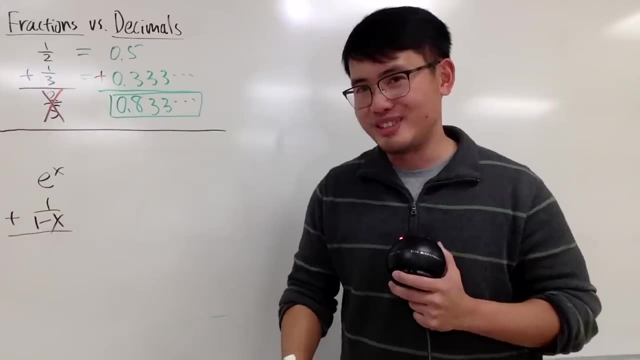 In that case, I seriously cannot even do the common denominator right. However, if you're willing to take these two functions and change them to polynomials, then you'll see. Let me just tell you guys the answers first. They both keep on going forever. 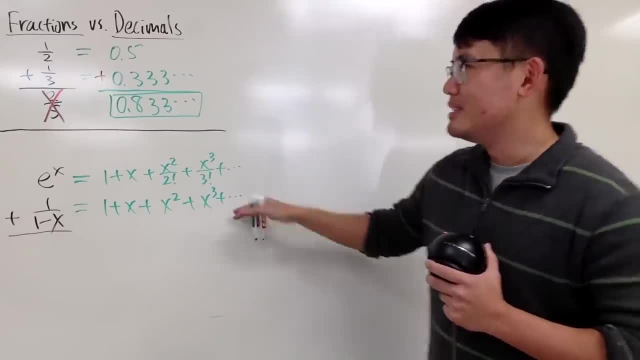 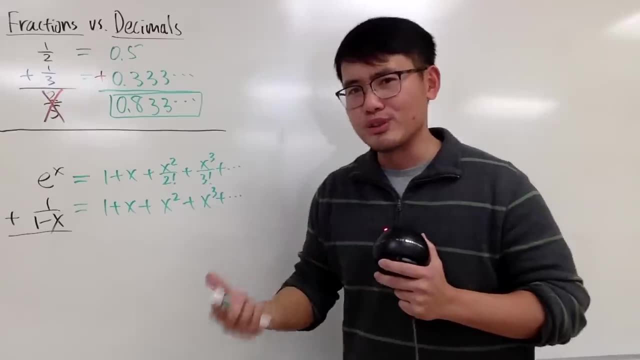 They do not end. That's why it's the infinite polynomial, So it's like the same idea of the 1, third. It keeps on going forever and depends on how many terms that you use and, of course, the more accurate the answer will be right. 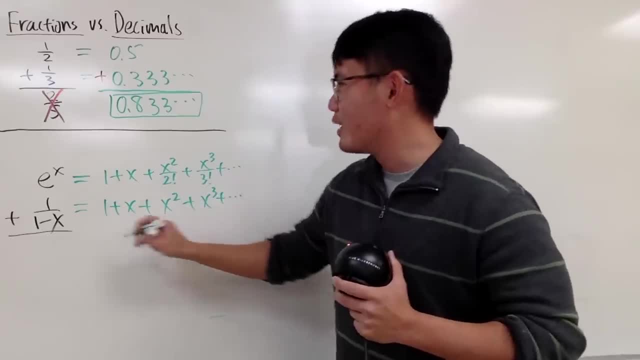 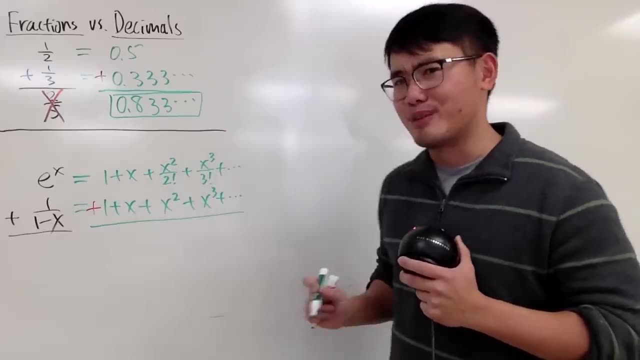 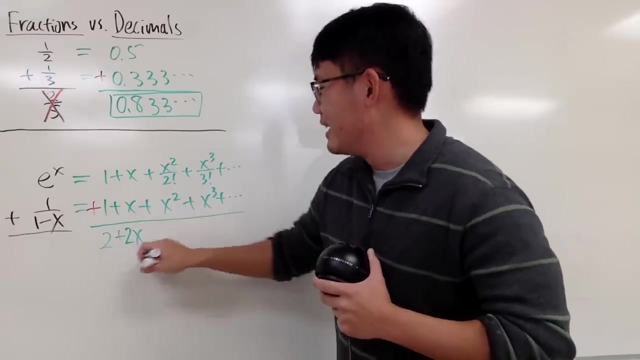 And if you look at this right here, wouldn't it be so much easier to add them up? Yes, because now we can just add them term by term. 1 plus 1 is 2.. Yes, I know. And then x plus x is 2x and plus. okay, 2 factorial means 2 times 1, which is 2.. 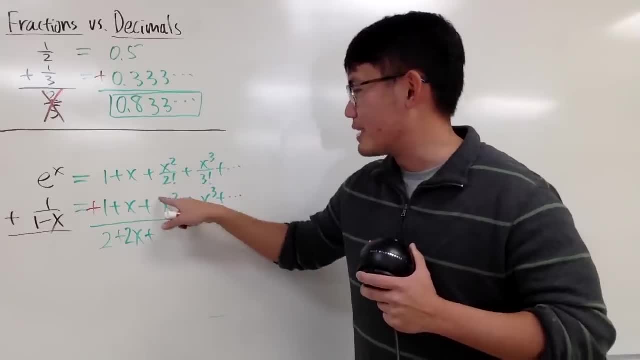 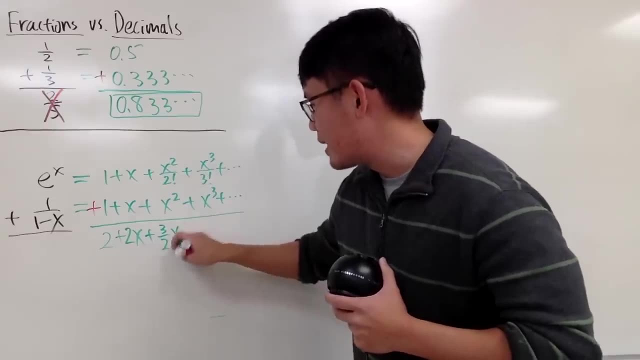 And this is in the denominator. so we have 1 half. We have to do 1 half plus 1. And you have to add the fractions legitimately. 1 half plus 1 is 3 half And you keep the same term, x squared. 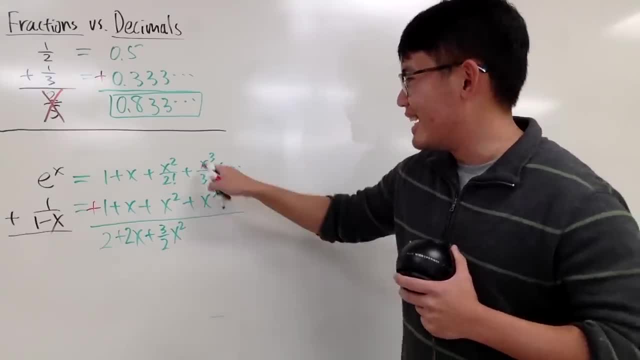 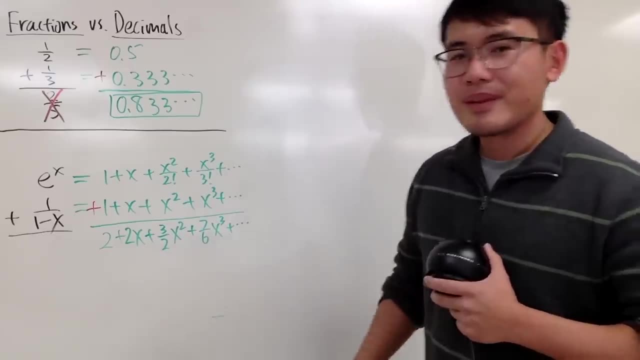 And then 3 factorial is 3 times 2 times 1,, which is 6.. And this is 1 over 6 plus 1, which is 7 over 6x. to the third power, plus dot dot dot. Guess what? 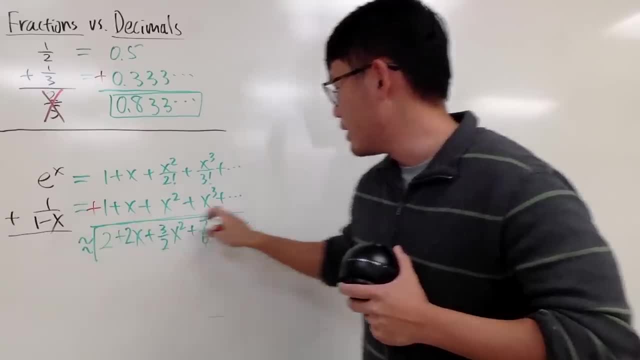 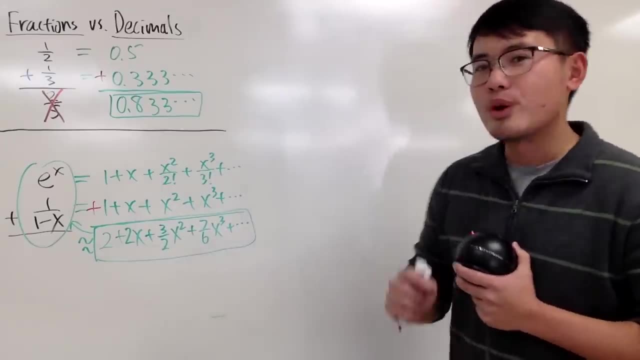 This right here will be a pretty good answer for this. if you want to add them up, Of course, I have to tell you guys more things, such as what we call the radius of convergence, And how exactly can we come up with this right? 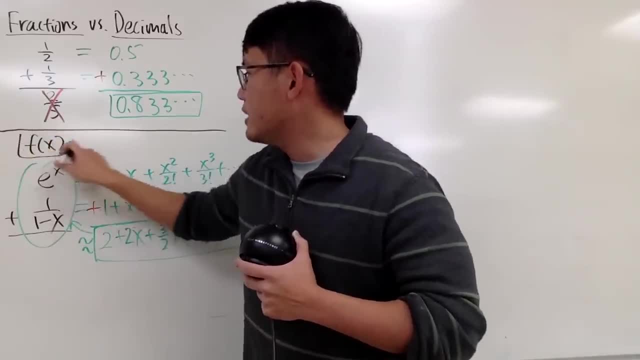 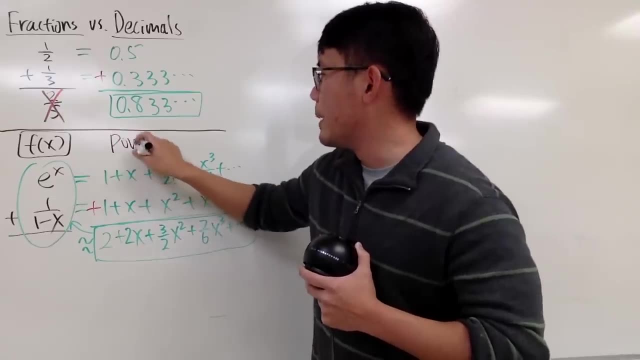 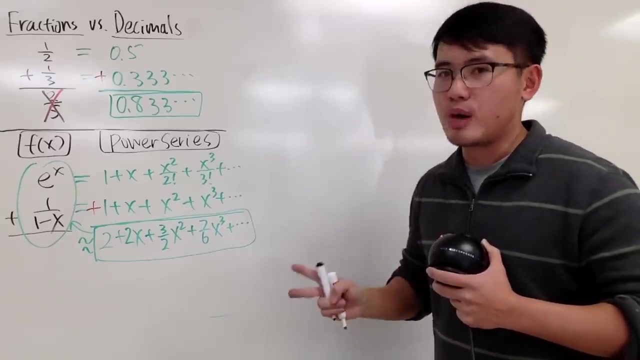 Anyway, here is the idea. Our goal is to write a rather complicated function, and we'll just write it as f of x, And this right here is what we call the power series, And you have two main ways to get the power series right, especially in Calc 2.. 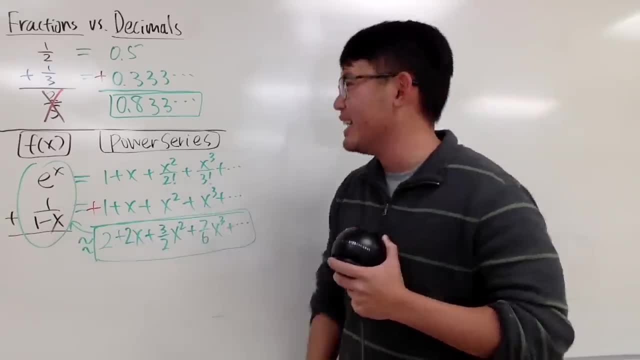 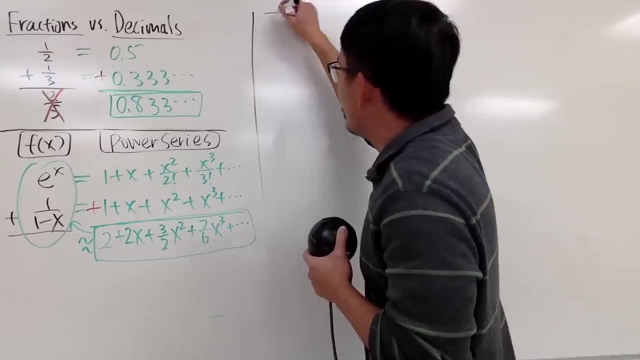 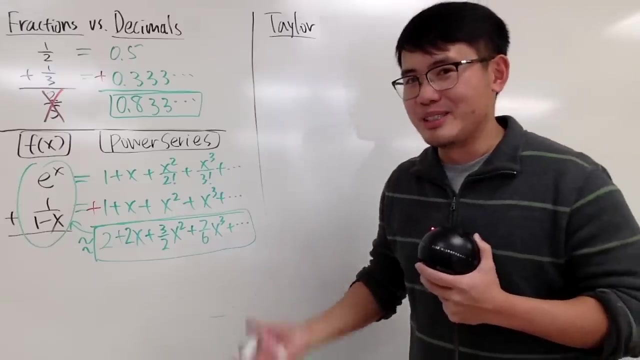 One is to use your best friend right And two, this right here is called the Taylor series, the Taylor formula, And when you use the Taylor formula, of course you want to be respectful to the answer that you get. So that's why you call this to be the Taylor series, because you use his formula. 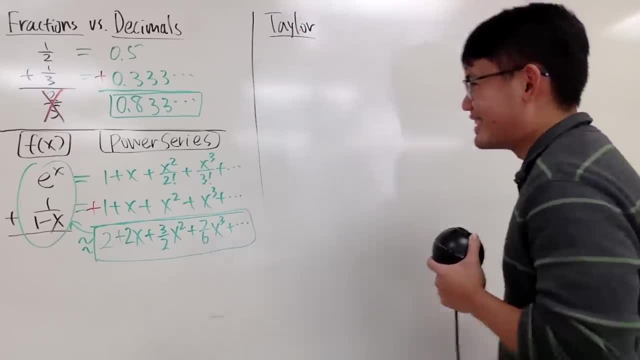 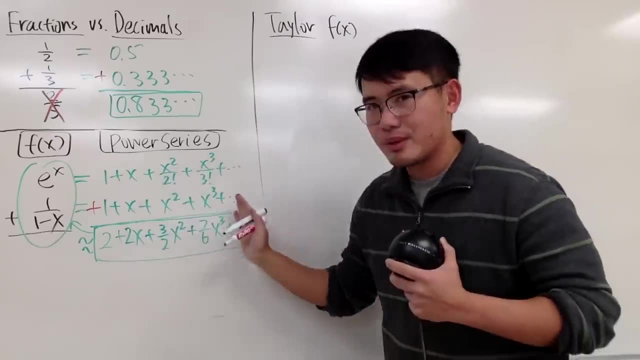 And I personally call this the dad if you're talking about the series. Anyway, let me write this down right here for you guys. First of all, our goal is to write f of x as an infinite polynomial, as a power series like this: 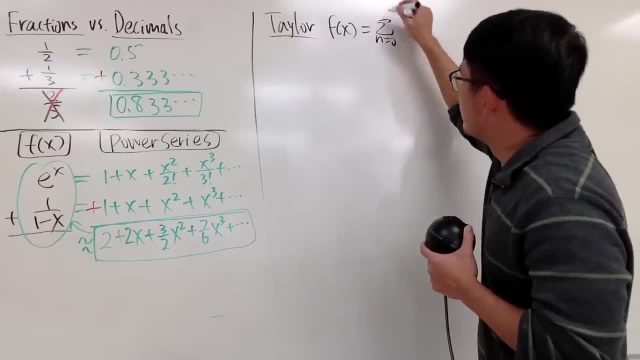 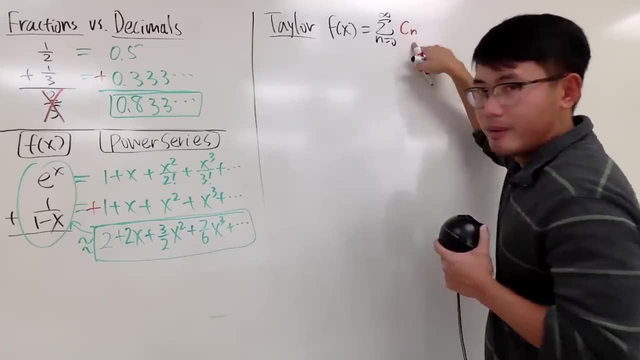 And I will write this down In the summation form. this is the sum, as n goes from 0 to infinity And the main goal is to figure out the coefficients. So I will just put down cn right here. This is the coefficient sequence. 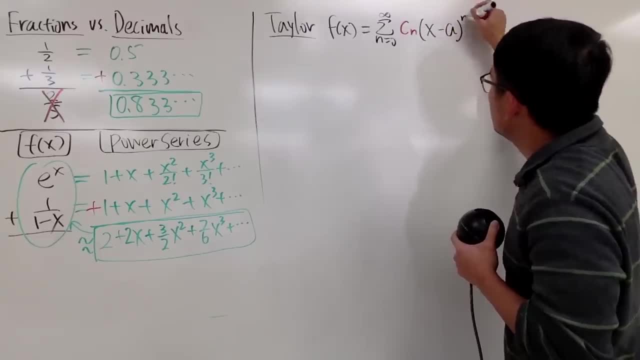 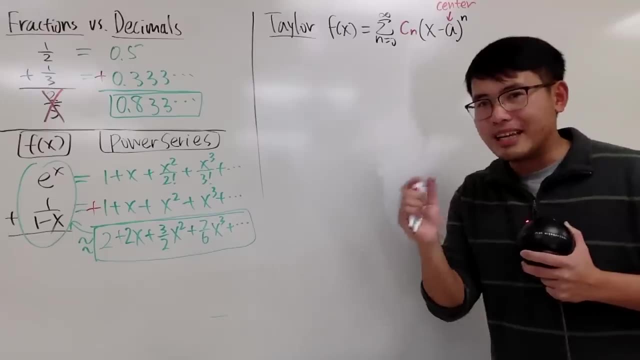 And then you have to write down x minus some number, a raised to the nth power. Well, what is a? a is what we call the center, So it's almost like the starting. It's your target number. Hold on, stop. 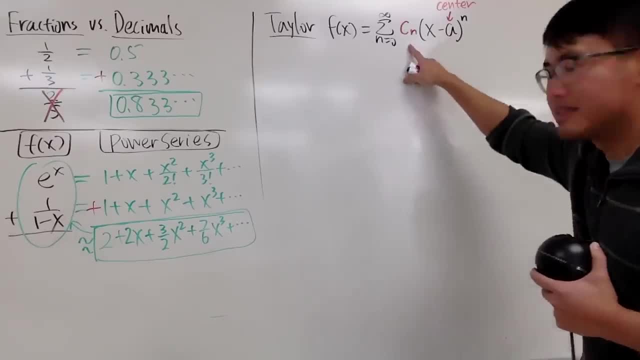 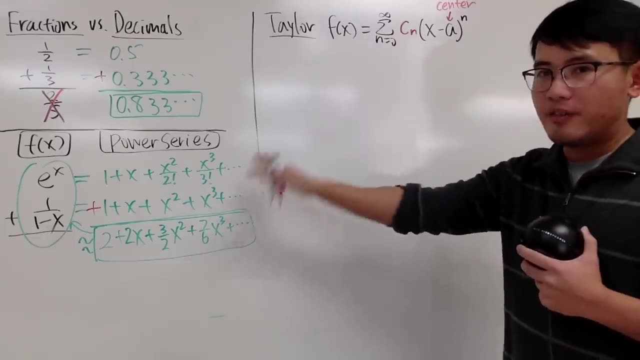 I will show you guys more later on with pictures, But I will tell you guys how to work Without the cn first. Well, right here, In fact, let me just write down the expanded version of this expression for you guys. All right, our goal is to figure out the c's. 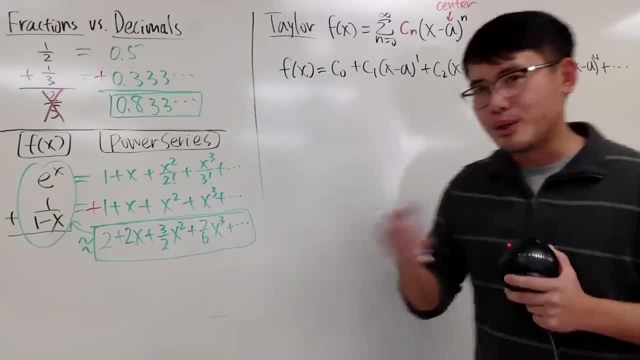 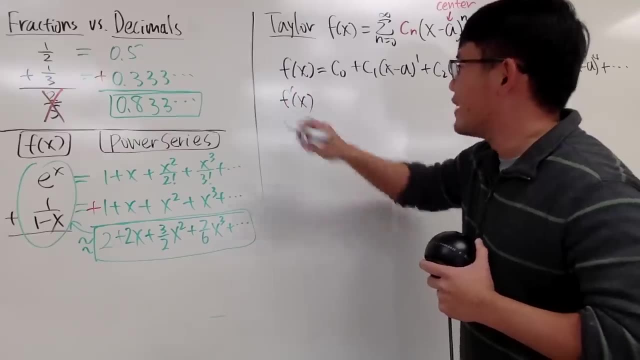 How can we do it? Well, you have a constant. How can you kill a constant? Yes, by integration. No, sorry, just kidding, By differentiations. So what we'll do is differentiate this one time, And in that case you'll see that c 0 will be gone, right. 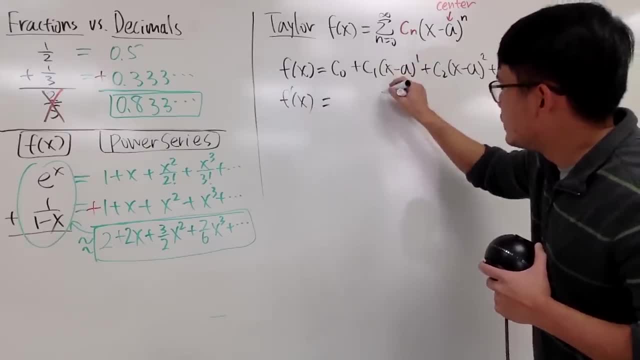 And when you differentiate this part, you just get the constant c 1. The relative of this is just 1.. So you just have c 1. And then when you differentiate this right here, you bring the 2 to the front. 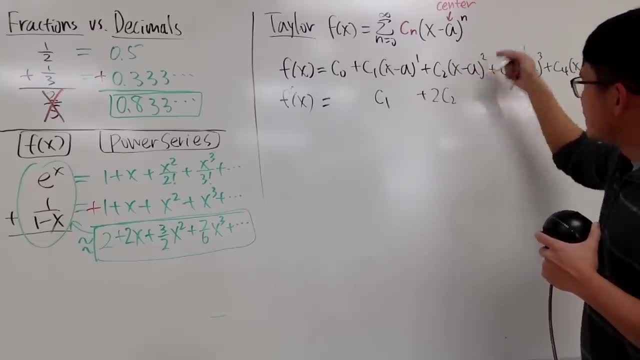 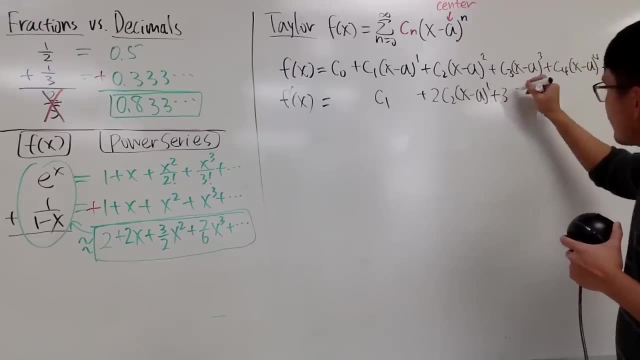 Don't forget about that. And then you have c: 2. And you minus 1. So you get c, You get x minus a to the first power, And you do the same thing: Bring the 3 to the front, 3 c, 3 x minus a to the second power. 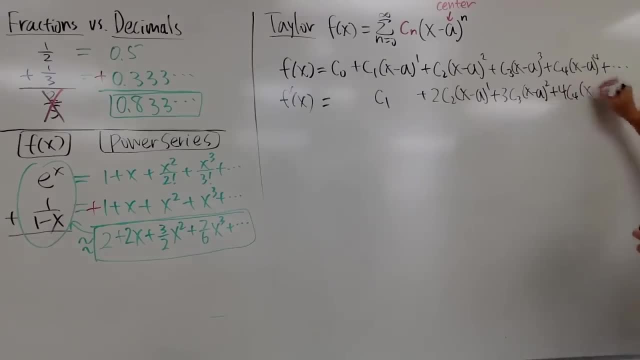 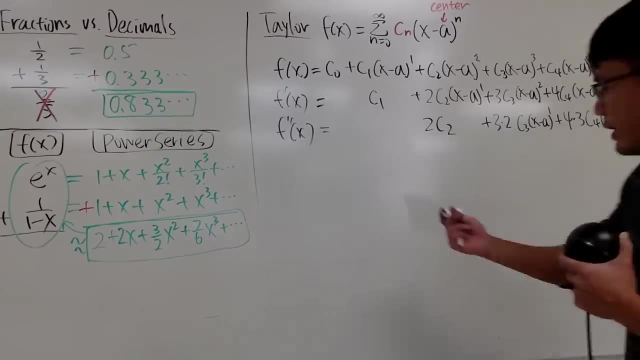 And then bring the 4 to the front, So you have 4 c, 4 x, minus a to the third power, And so on, so on, so on. So that's cool, And now let's just differentiate again. Well, let's do it again. 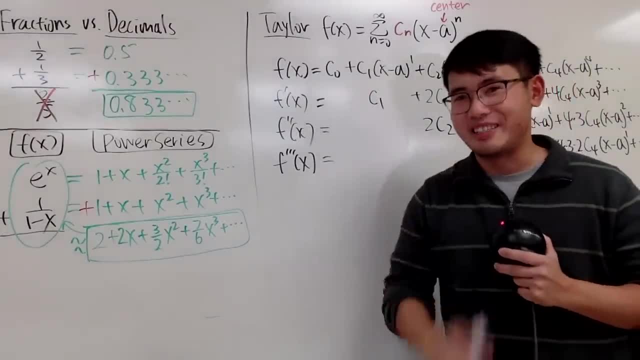 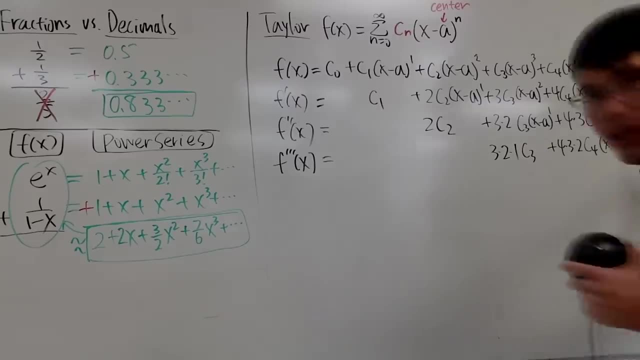 Let's look at the third derivative, namely the jerk of that. No, just kidding. Let's see. Hey, I see this is x minus a to the first power, And you have more x minus a terms later on, right, Because you can see that this is x minus a to the first power. 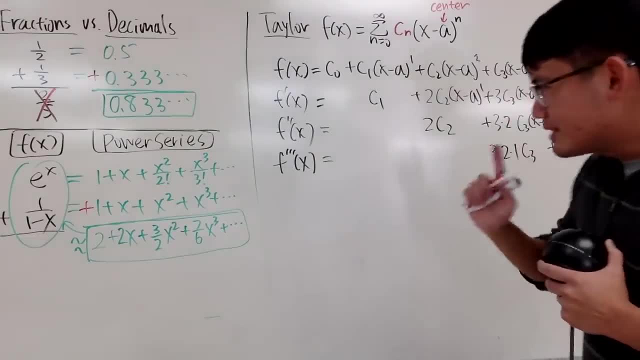 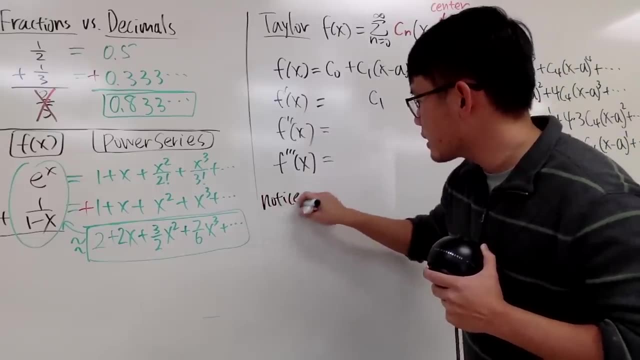 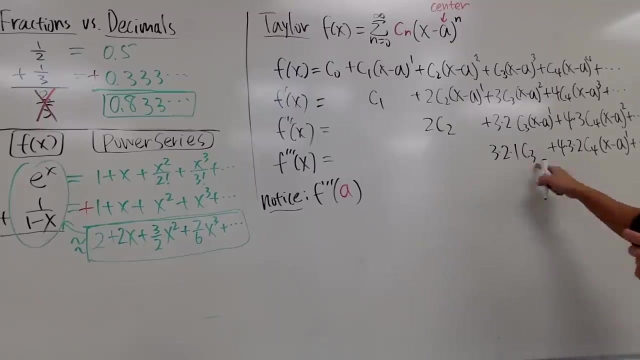 And the next term you have x minus a to the second power. So the smart number to use is that we can just plug in a for x. So I will just tell you guys notice, if you put a into x. well, this right here is just a constant term. 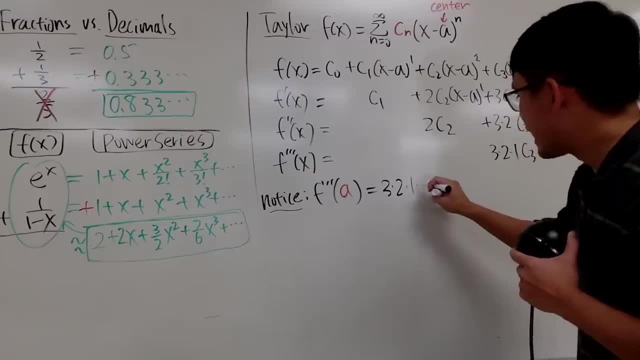 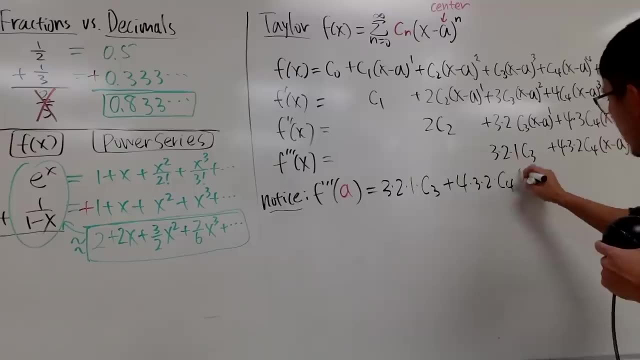 So this right here stays, which is 3 times 2 times 1 times c, 3.. And this right here it's going to be plus, 4 times 3 times 2 times c, 4 x, which is the a now. 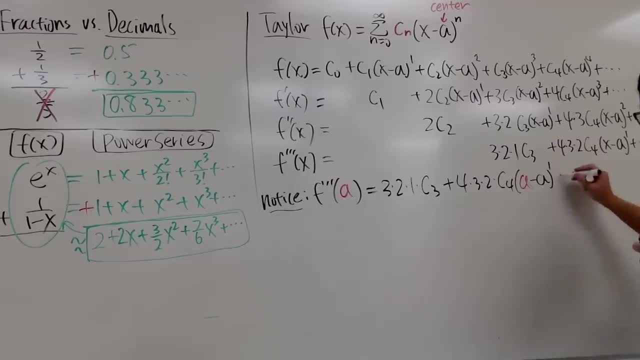 But we are minusing the a to the first power, And then this right here- it's actually a dandillo because it's just a zero- And in fact all of them, they all have a minus a to some power. 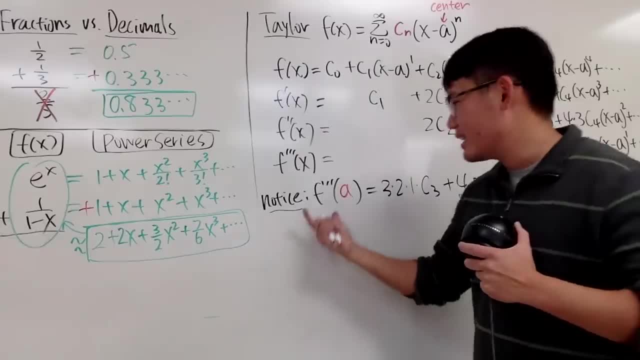 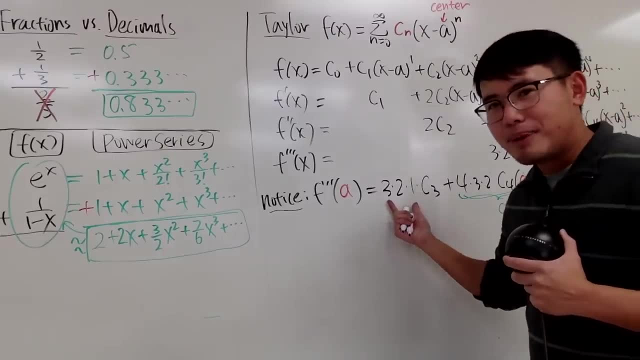 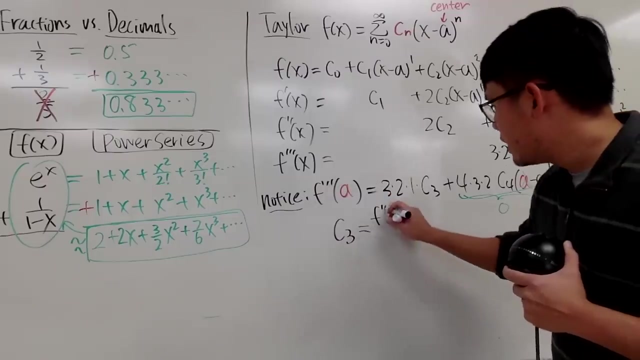 So everybody right here will be zero. So if you look at the third derivative of a, it's just this. So how can we solve for c 3? We can just divide it by 3 times 2 times 1 here. So in another word, note: c 3 is just the third derivative of the function.